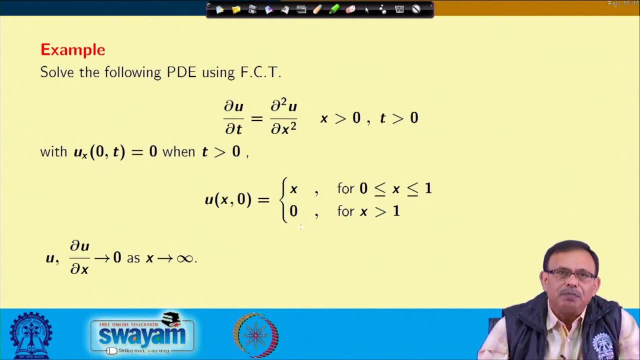 u and del u del x approaches 0 as x approaches infinity. So from the given condition again, del? u del x approaches 0, u x 0, t is 0 is given, u x 0 is given. Therefore I have to apply. 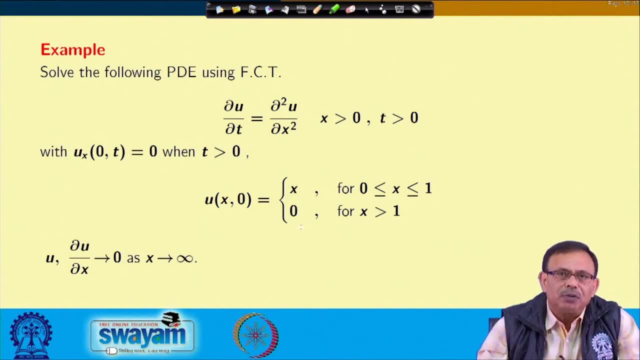 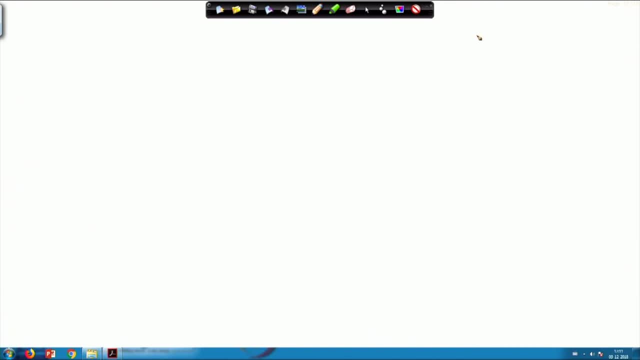 the Fourier cosine transform With respect to the variable x, not with respect to the variable t. So your equation here again was: del u del t equals del u del t equals del del 2 u del x square. So if you apply Fourier cosine transform with respect to x on the given equation, So you will obtain: 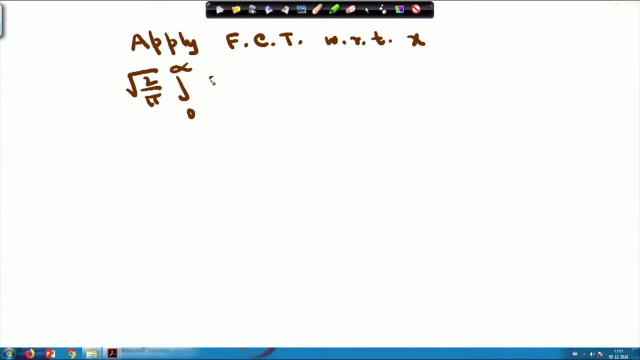 root over 2.. 2 by pi 0 to infinity del u del t into cos of alpha x d x. This is equals to root over 2 by pi 0 to infinity del 2 u del x square into cos of alpha x d x, which gives d d t. 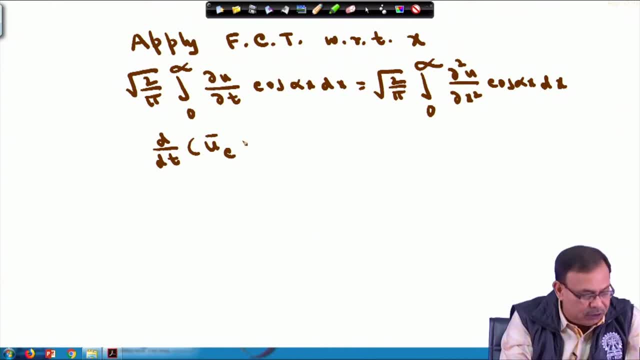 of u bar c, Left hand side will be nothing but 0 to infinity. u cos of alpha x, d, x, which is again u bar c, And on the right hand side again, if you integrate you will obtain root over 2 by pi del u del. 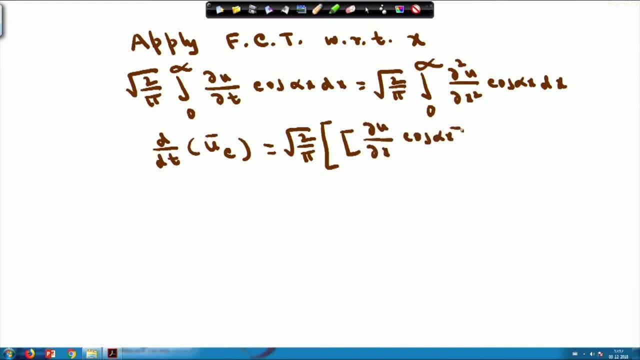 x into cos of alpha x, 0 to infinity, plus alpha into 0 to infinity. del u del x into sin of alpha x, d, x And further. please note that del u del x it is given two things: One is u x 0, t is 0 and. 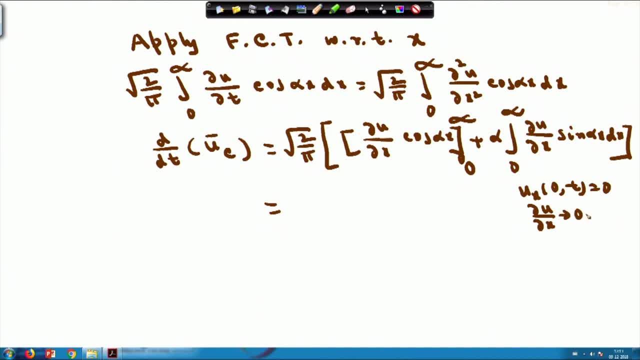 del u del x approaches 0 as x approaches infinity. These two conditions are provided: u x 0, t equals 0 and del u del x approaches 0 as x approaches infinity. In fact, what do we have here? those terms are denoted as 0 as x approaches infinity. Now I will one more viewgate. let us see. 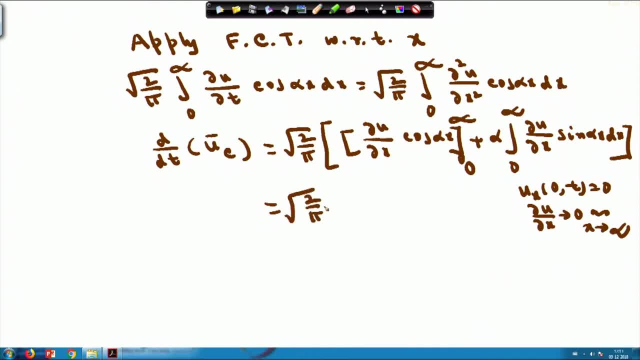 what we have to do in case the composition throws it over. So first part is the number of derivative, that is, the particular iteration of the union of alpha to infinity, which is equal to minus lambda. t mio~ del u x. 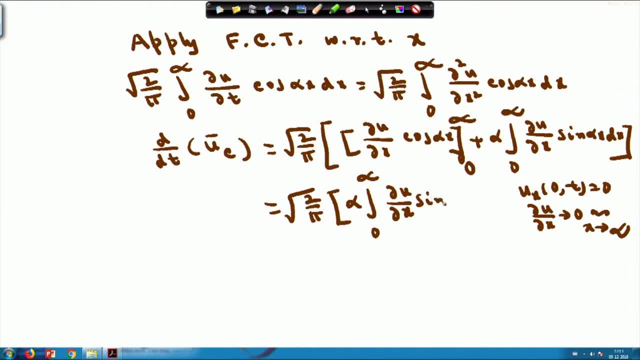 So if you substitute these two values, then this particular term will vanish. you will have only the second integral, that is root over two, by pi into alpha, into 0, to infinity, del u, del x into sin, of alpha x into dx. Again, you break it. you will be the same formula. 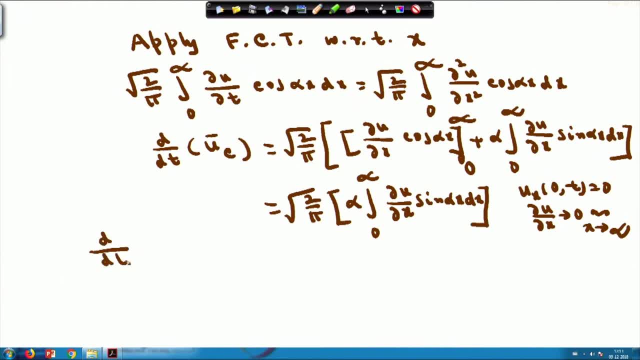 So this bulk will get in the numerator, and numerator should also be equal to開心 that break it. you will obtain d d t of u bar c. This will be equals to root over 2 by pi, alpha into u sin alpha x, 0 to infinity minus alpha square into 0 to infinity, u cos of alpha x. 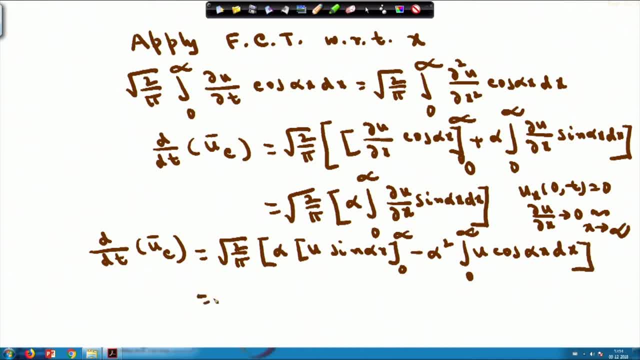 d, x, and this value will be equals to minus alpha square u bar c, with the condition that u approaches 0 as x approaches infinity. We know this thing: u approaches 0 as x approaches infinity. therefore, this value, this term, will vanish. this term will vanish and the next. 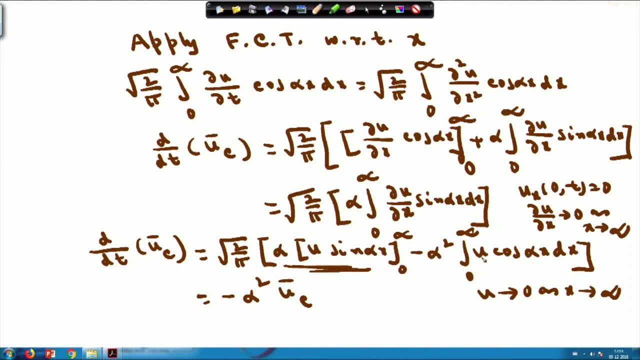 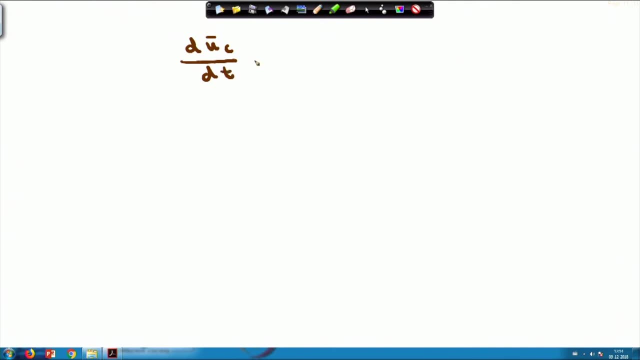 term alpha square into root over 2 by pi 0 to infinity. u bar c into alpha square, into u cos of alpha x. d x is nothing but u bar c, So that your equation, differential equation, becomes d? u bar c, d t plus alpha square, u bar c. this is equals to 0 and the solution: 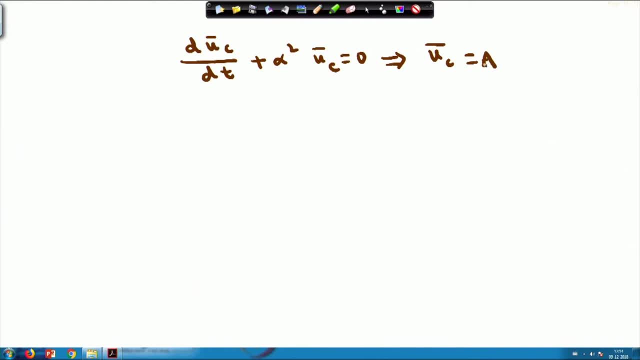 of this one is u bar c equals a into e power minus alpha square t. I have to find out the value of the constant And a. now using the similar process, that is, at t equals 0, what is the value of u bar c? 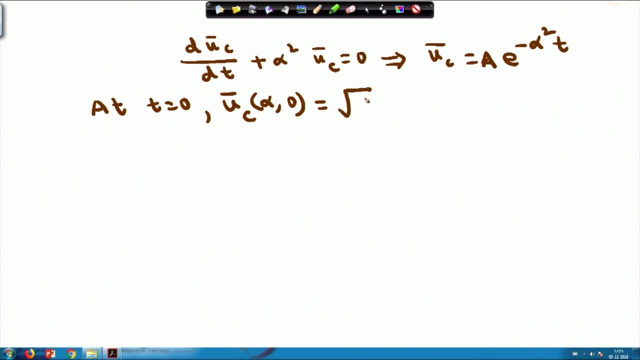 alpha 0 from the definition this equals: you can write down root over 2 by pi 0 to infinity. this is nothing but u x 0 into cos of alpha x d x, because u bar c is this So cos of alpha x d x. 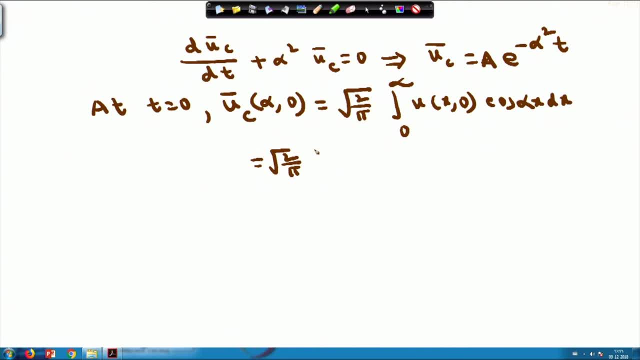 So u bar c is the. this is: this is the: u x, 0 a x. it is given from 0 to 1.. So it is: u x 0 equals x, cos of alpha, x, d, x. So u bar c is nothing but the Fourier cosine transform. 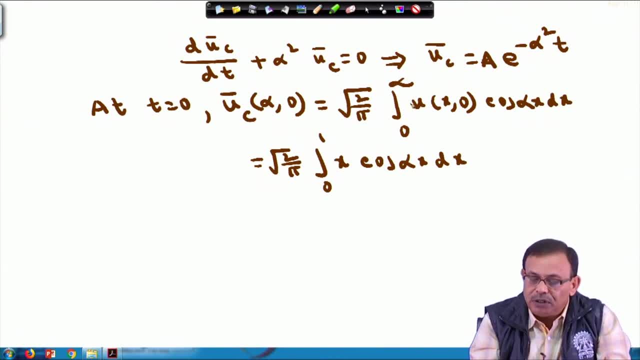 of the function u x 0 for that region. we have written 0 to infinity, u x 0. cos of alpha x, x into root over 2 by pi is u bar c alpha 0. Now u x 0 is 1 in 0 to 1. u x 0 is x and. 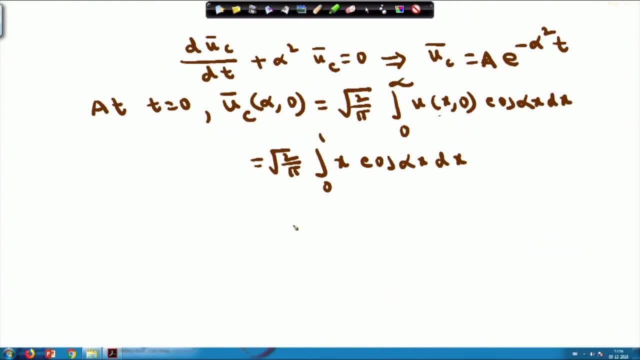 otherwise it is 0. So that you will obtain 0 to 1 this thing. If I evaluate this integral, you will obtain: root over 2 by pi x, sin of alpha x by alpha minus 1, by alpha square into minus cos of alpha x, 0 to 1.. If I evaluate the limits, then 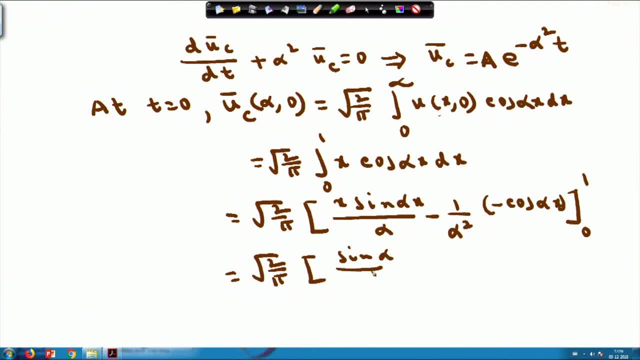 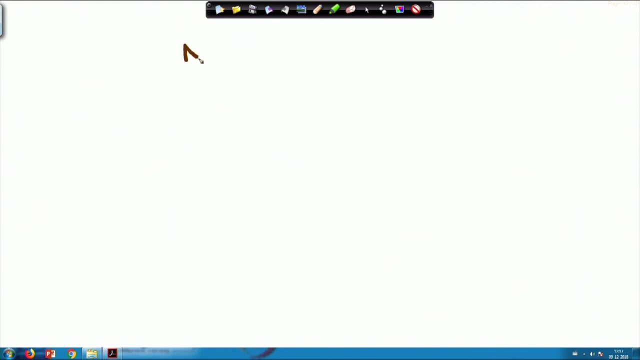 ultimately, I will obtain sin alpha by alpha plus cos alpha minus 1 by alpha square. So once I am obtaining this, therefore, if I substitute it in the given equation, this e power term will vanish. So your a will become this term only. that is, your a is now from here. if I substitute: 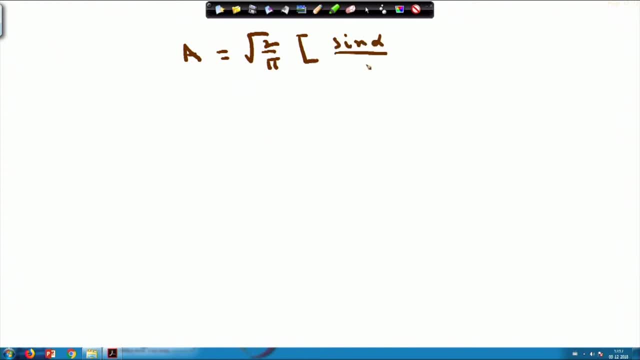 root over 2 by pi, sin alpha by alpha plus cos alpha minus 1 by alpha square. So u bar c. this will be equals to root over 2 by pi into sin alpha, by alpha plus cos alpha minus 1, by alpha square into e power minus alpha square t. And once I obtained u bar c I can. 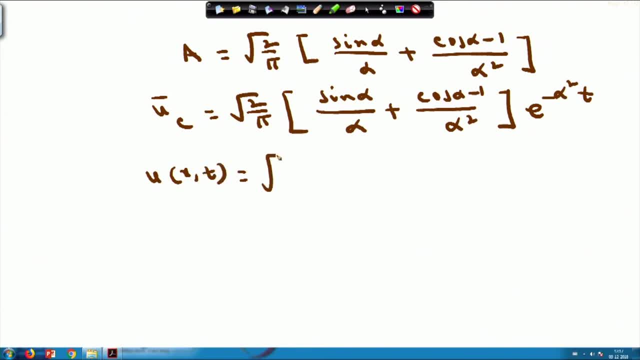 always write down u x t using the inversion formula: root over 2 by pi, 0 to infinity. u bar c into cos of alpha x into d alpha And you put the value of u bar c- u bar c is your root over 2 by pi- into root over 2 by pi. will come here then sin alpha by alpha plus cos. 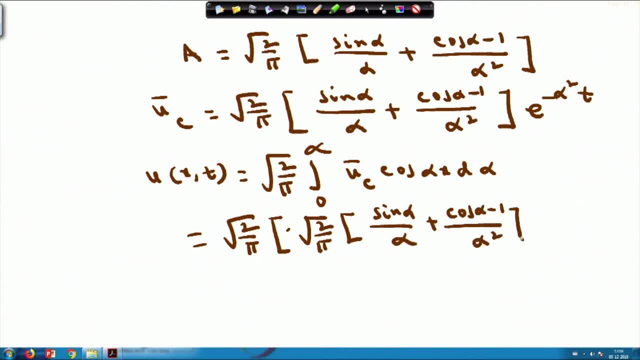 alpha minus 1 by alpha square into e power minus alpha square, t into cos of alpha x into d alpha, And I can evaluate the, the integral, to obtain the value of this one. sorry, one thing I missed, that is: this is from 0 to infinity, the integration from 0 to infinity, So u x. 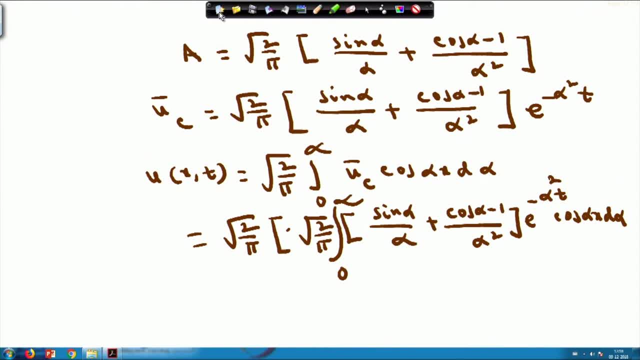 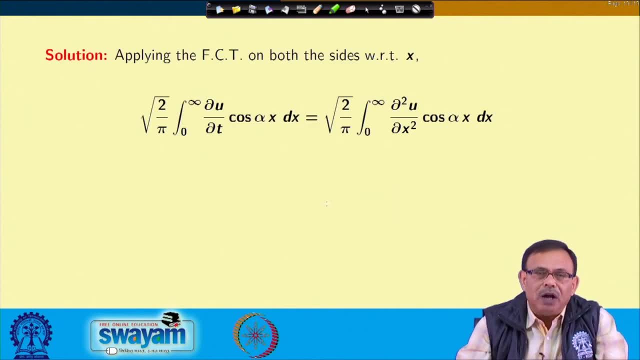 t. is this integral? if I evaluate it, I will obtain the result. Let us see quickly over here. the problem was given as this one. So what I am doing, I am just taking Fourier cosine transform, then, using the earlier methods, I am evaluating the integral and in evaluation of the limit we are using the condition u x 0, t is 0 and. 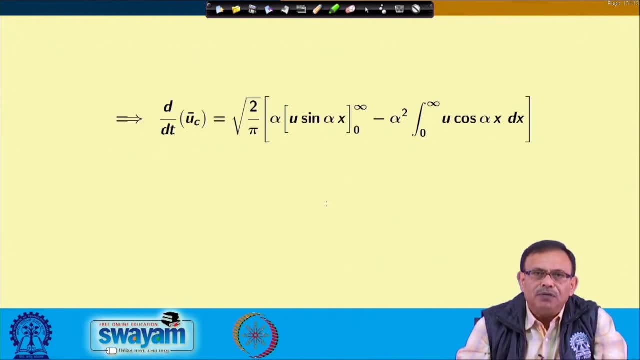 del u del x approaches 0 as x approaches infinity. So that, again evaluating, I am ultimately obtaining my ordinary differential equation as d? u bar c, d t plus alpha square u bar c equals 0.. So the solution is: u bar c equals a? e power minus alpha square t. So I have to find out. 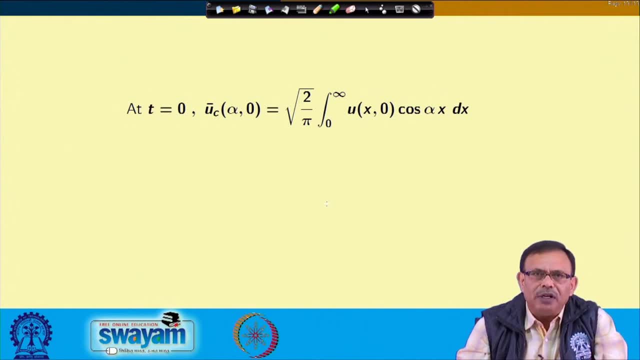 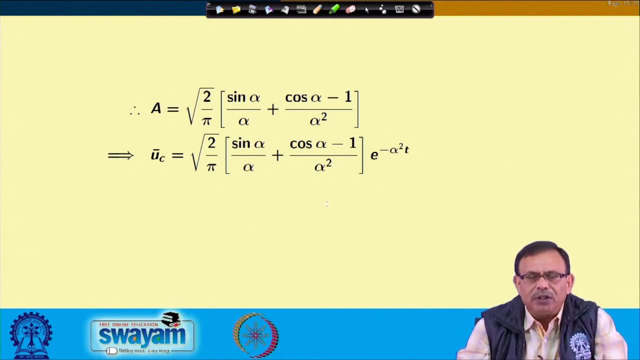 x d x and you can substitute the value of u bar c cos of alpha x d, x and you now can write down the integral. all those are directちら pre extended a. I can find out u bar c as a function of alpha and t and from here I can write down: u x t is equals to root over 2. 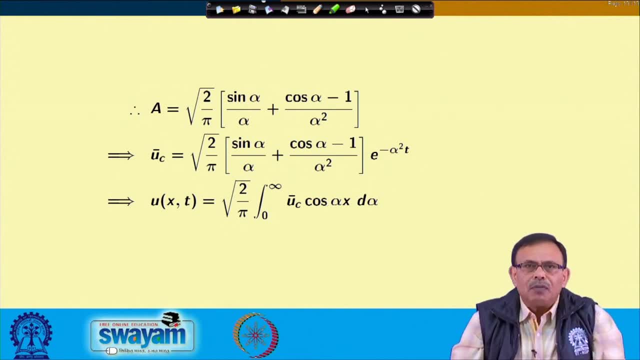 by pi 0 to infinity into u bar c, cos of alpha x, d, v, x, and you can substitute the value of u bar c over here and you will obtain the required integral. if I evaluate the integral, I can find the value of u x t. 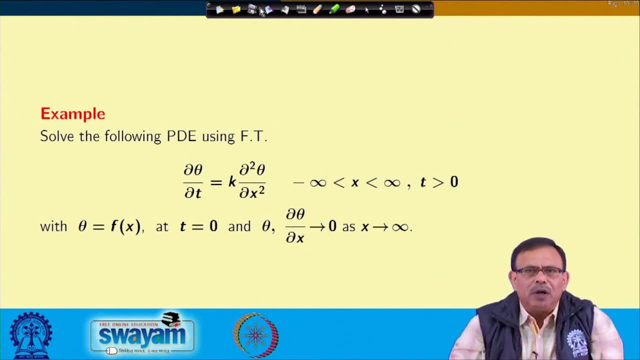 Let us see the other one. till now, whatever problems we have done, that is, using Fourier sine transform or Fourier cosine transform. Now let us solve another problem using Fourier transform. The function is given as: del theta del t equals k del 2 theta del x square x. 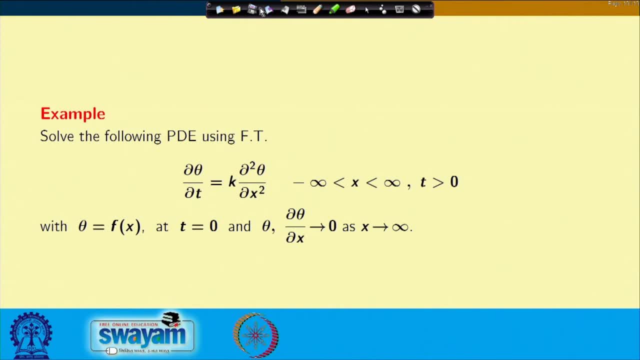 lies between minus infinity to infinity, t greater than 0 here, and with theta equals f, x at t equals 0, and theta and del theta del x approaches 0 as x approaches infinity. So theta equals f, x at x, t equals 0. we have assumed means the result whatever I will obtain. 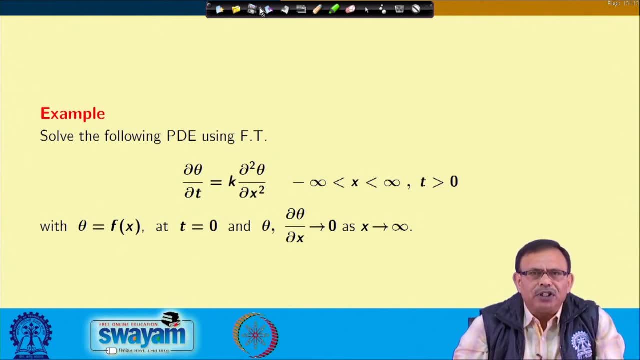 that I will obtain in terms of f x only, and if I substitute the f x by a particular function, I can evaluate the value. So the general function we have used to it as f x. Now, if you see the problem itself here, I have two variables, x and t. t is given. 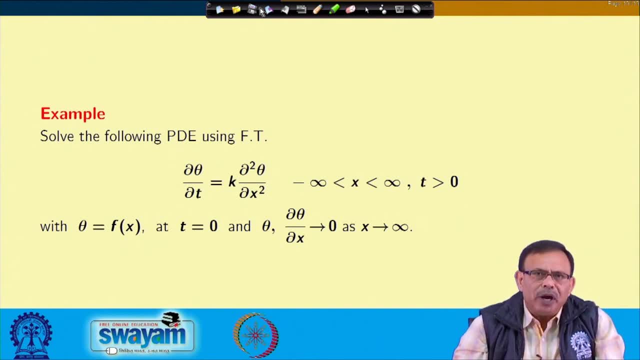 as greater than 0 and x lies between minus infinity to infinity, and you know the range for Fourier transform is from minus infinity to infinity. Also, it has been given that del theta del x approaches 0 as x approaches infinity and theta also approaches 0 as x. 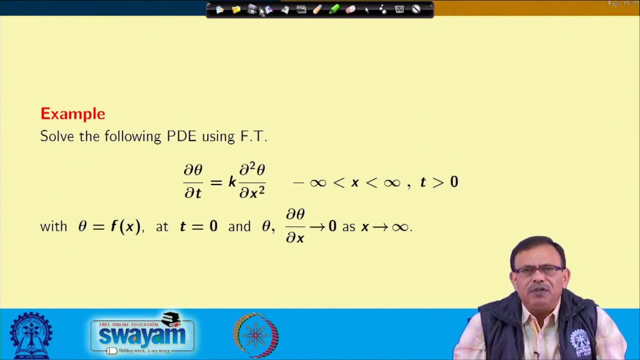 approaches infinity. Therefore, the from the given criteria we can tell that I have to use the Fourier transform on this given equation with respect to the variable x, not with respect to the variable t, because range of t is from 0 to infinity, not from minus infinity to infinity. So we 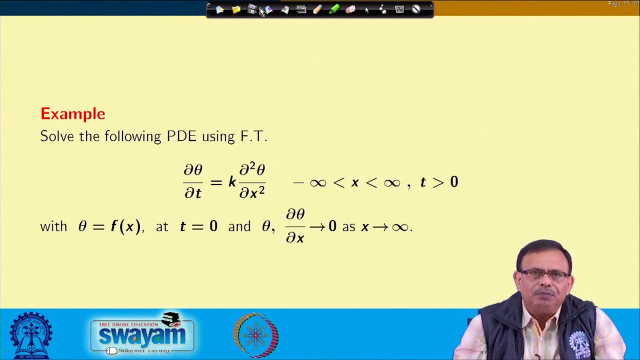 should be careful. whenever we are trying to solve a problem, The first thing I have to think which transform I can use Just the first thing. when we are solving a problem, the first thing I have to think which transform I. 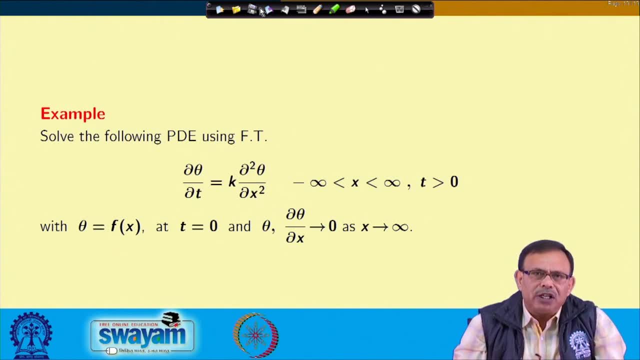 I can use Here. just like, since x varies from minus infinity to infinity, I can take the Fourier transform because the conditions are also given. but I cannot use Fourier transform with respect to the variable t, because range of t is from 0 to infinity. 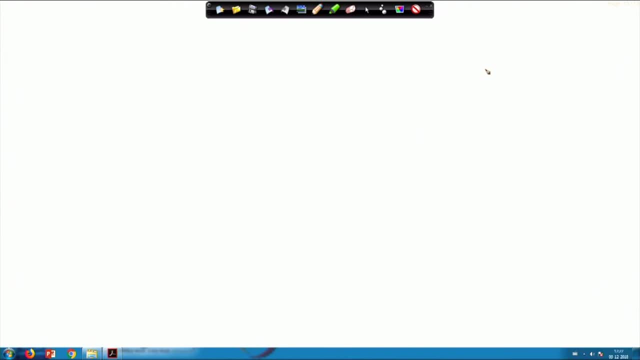 So to solve the problem, basically, your equation has been given as del theta del t. this is equals k into del 2 theta del t square. So apply Fourier transform on both side. if you apply Fourier transform with respect to the variable x on this given equation, So left. 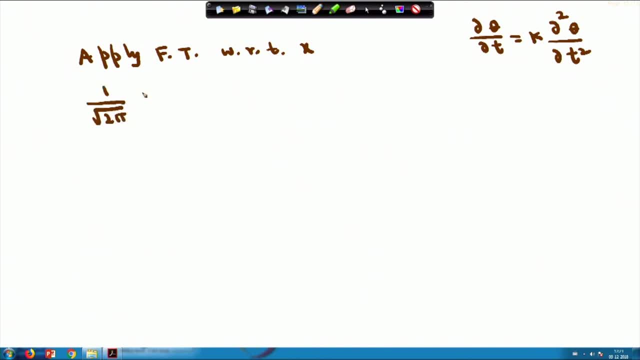 hand side will be 1 by root, 2 pi, from the definition minus infinity to infinity del theta del t Into e, power, i, alpha, x, d, x, so that it will be a function of x and right hand side will be k into 1 by root over 2 by pi, minus infinity to infinity del 2 theta del x square into: 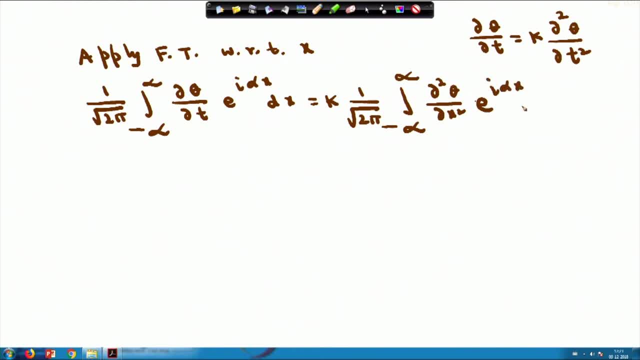 e power into e power, i alpha x into d x. Now, if you see here the left hand side del del t, Where this function is a function of alpha and x. So therefore, del del t you can bring outside, and once you are bringing outside, I can make it d d t, So your integral becomes. 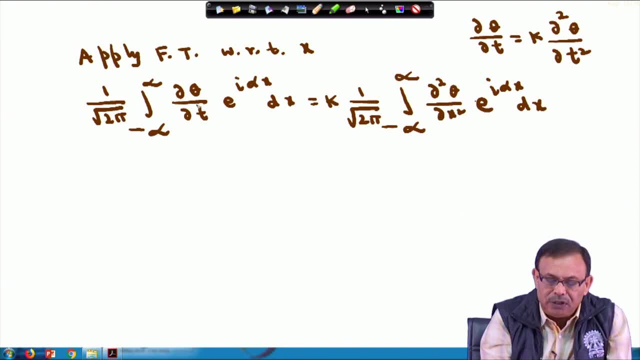 then 1 by root, 2 pi minus infinity to infinity, theta e, power i, alpha x, d, x, and this is nothing but the Fourier transform of theta, So that the left hand side you can write down d d t of say theta bar, And where theta bar is nothing but the Fourier transform of the function theta, which I am. 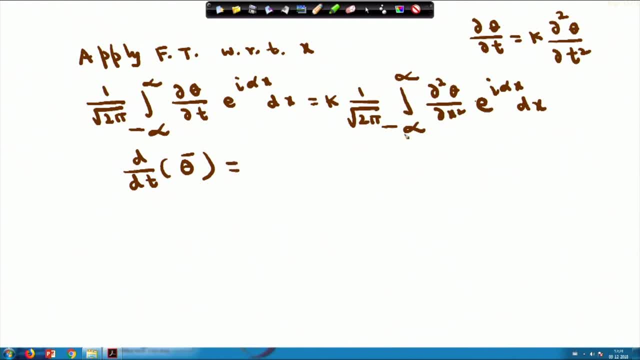 denoting as this And right hand side. now I have to use the integration by parts and I have to find out the value k into 1 by root over 2 by pi. First term will be del theta, del x into e, power i, alpha x minus infinity to infinity d x. So this is the integral. 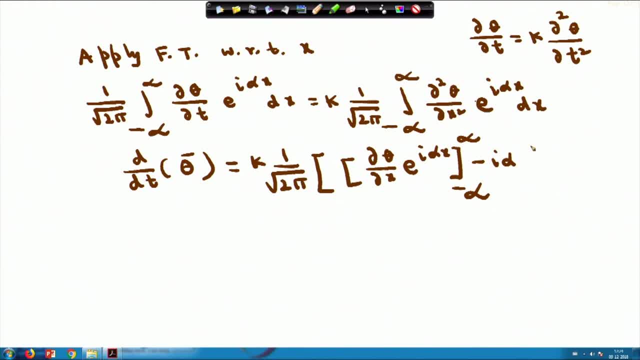 infinity minus i alpha will come over here- minus infinity to infinity. del theta del x into e power i alpha, x into d x. Now this, please note- that del theta del x approaches 0, it is given del theta del x approaches 0 as x approaches infinity. So therefore, in 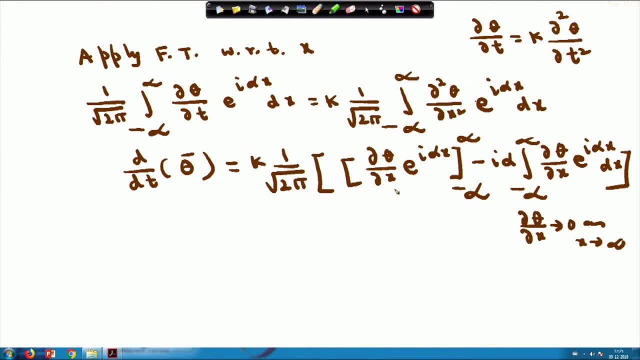 using this part, And this is also using this condition- this value, as x approaches infinity or minus infinity, this term will be vanishing. So we will have only this term minus. i alpha into k will come i alpha k by root over 2, by pi minus infinity to infinity. e power i alpha x into del theta. 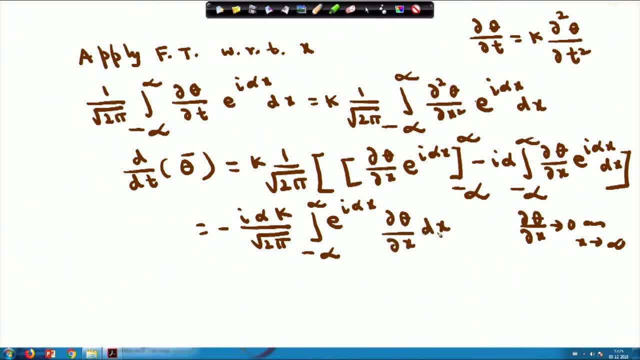 del x into d x. And this again, if you evaluate the integral you will obtain this equals minus i alpha k by root over 2 by pi into here it will be theta into e power i alpha x minus infinity to infinity, minus i alpha into minus infinity to infinity. So this will be the integral. 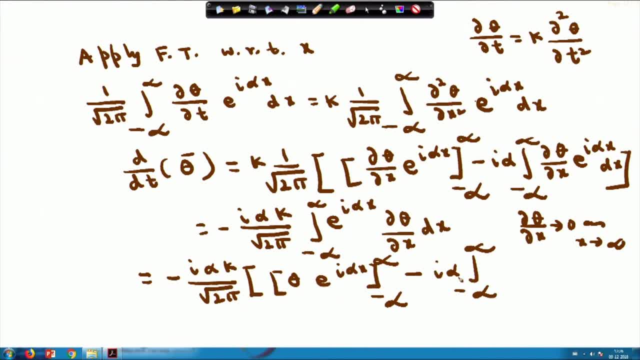 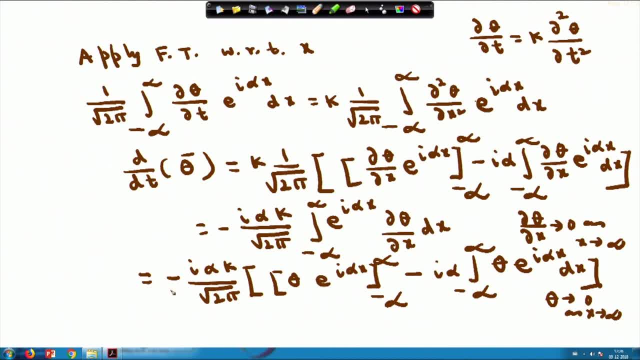 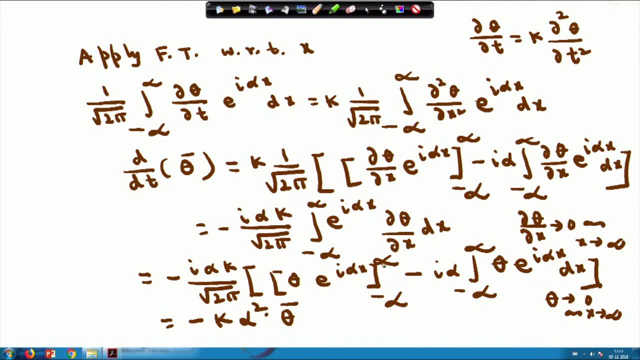 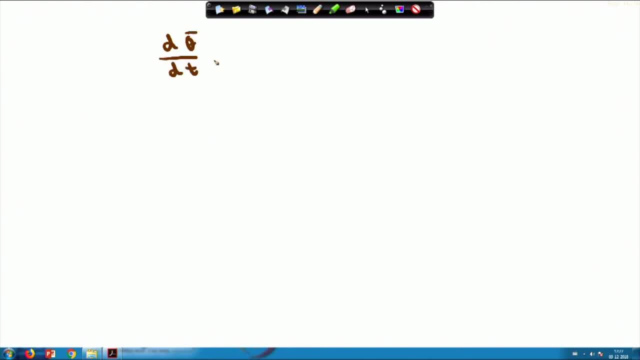 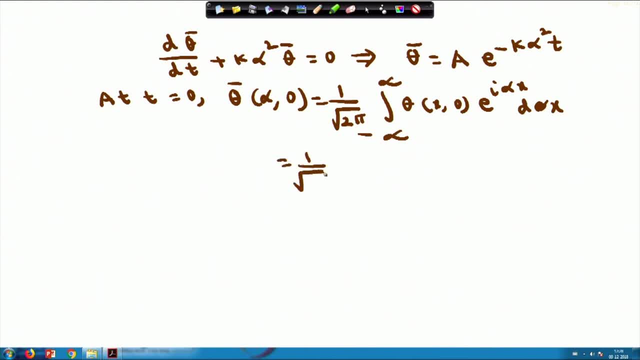 So this equals 1 by root, 2 pi minus infinity to infinity. theta x 0 is nothing but has been given as theta x 0 is here f x, so f x into e power, i alpha x, d x, And if you see, 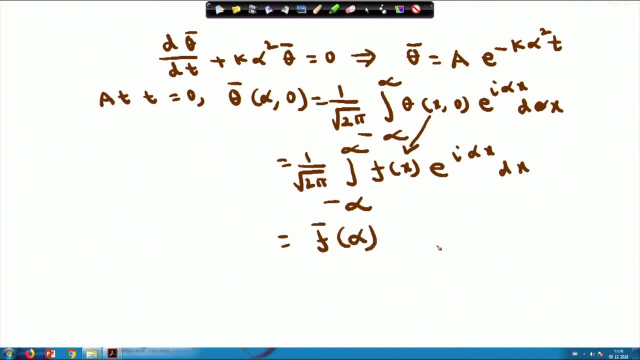 this you can tell as f bar alpha, where your f bar alpha is nothing but the Fourier-transform of the function f x. transform of the function f x. So ultimately you are getting theta bar alpha 0 equals f bar alpha where f bar alpha is Fourier transform of f x. If f x is known to me, then I can. 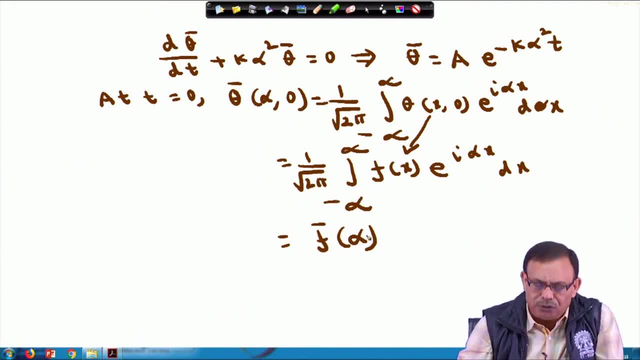 calculate what is the f bar alpha also. So by using this, if I put it on this particular equation now this value, I will obtain my a as f bar alpha. So once I am obtaining my a as f bar alpha, then I can write down my theta bar equals. 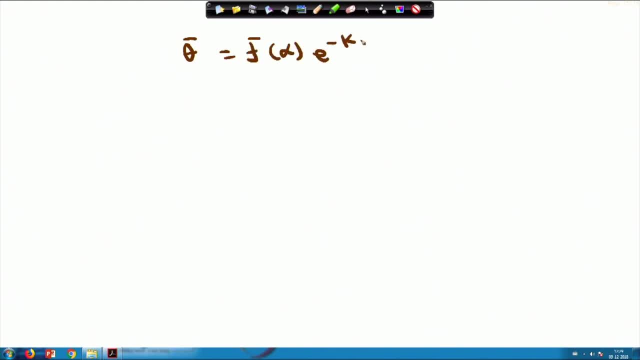 f bar alpha into e power minus k alpha square t, So that from here you can write down, from here you can write down theta x, t. using the inverse Fourier transform. This equals 1 by root over 2, pi minus infinity to infinity. 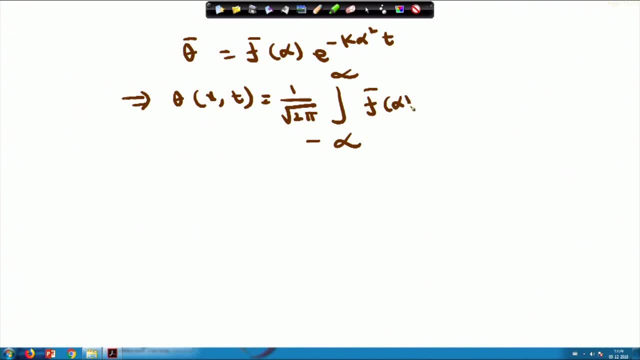 So your f bar alpha e power minus k, alpha square t into e power minus i, alpha x into d alpha, I will obtain this thing And if f bar is known to me, then I can evaluate this integral. So by this way we can find out the value of theta x, t. So let us see. 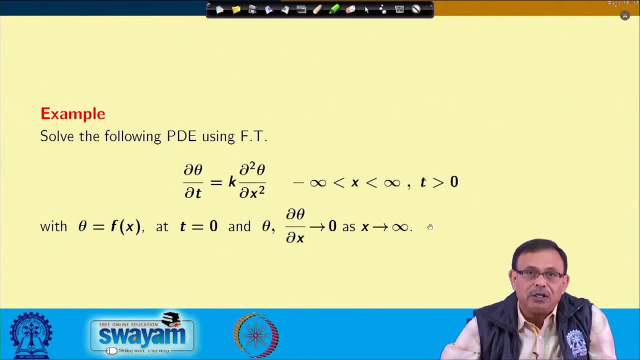 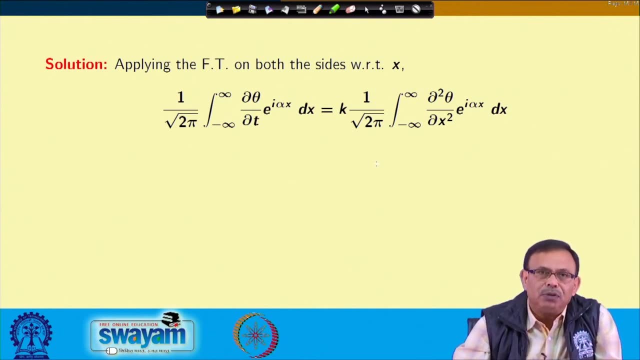 quickly over. here The problem is given as like this: So I am taking the Fourier transform 1 by root, 2 pi minus infinity to infinity del theta. del t equals e, power, i, alpha, x, d, x, And the right hand side is this, Left hand side is nothing but d d t of theta bar, because you are taking 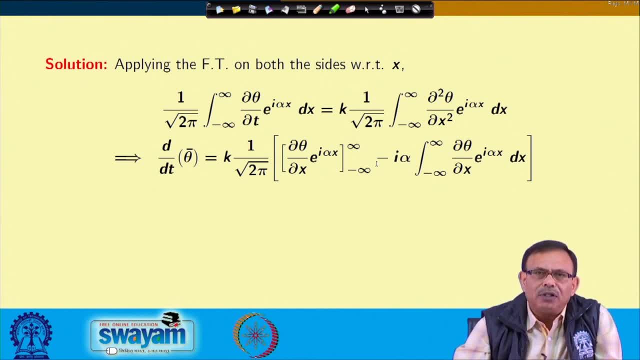 the Fourier transform with respect to x And for the right hand side you have to evaluate the integral And by substitute you can write down the value of theta x t into e power minus x t plus e power x t And as you substitute del, theta del x approaches 0 as x approaches. 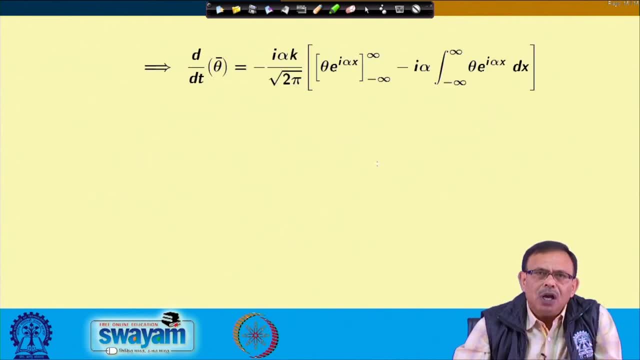 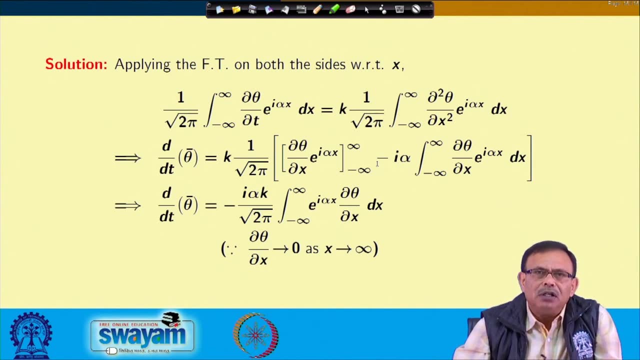 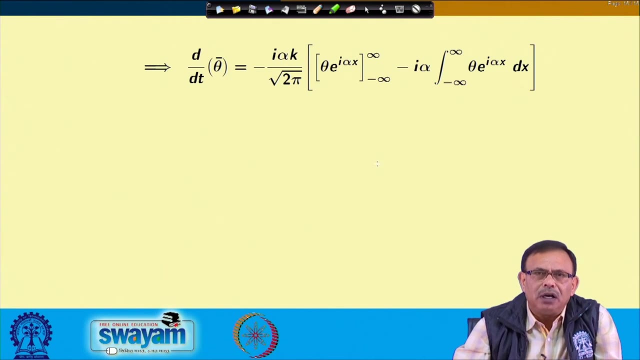 infinity. I can find out the solution. And as theta x approaches 0, as x approaches infinity, then the limiting value of the first term will be 0. So that I will have only the second integral. Now, second integral: again, I am evaluating by using integration by parts, and then this: 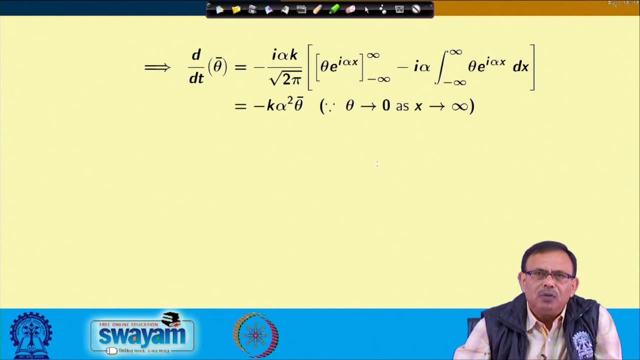 ultimately becomes minus k alpha square t into e power minus alpha times the right hand, theta bar, where theta approaches 0 as x approaches infinity, is given to us. So I am getting the differential equation like this, whose solution is: theta bar equals a e power minus. 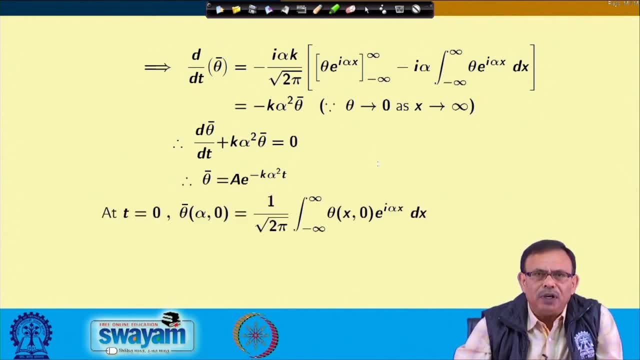 k alpha square t. So I have to find out: the value of a at t equals 0, q bar alpha 0. this is equals 1 by root, 2 pi minus infinity to infinity. theta x: 0 into e power i alpha x. 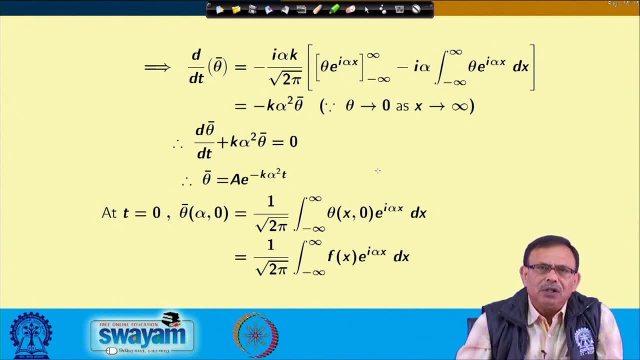 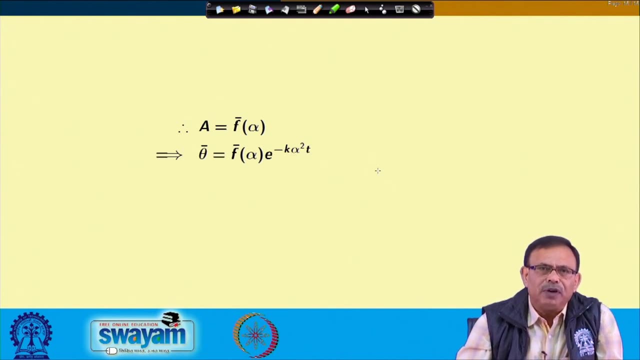 So theta x 0 is known as f x, So that I will obtain this, and this is nothing but f bar alpha, that is, Fourier transform of the function f x. Therefore, your value of a will be f bar alpha. and once I am obtaining f bar alpha, I can find out the theta bar equals. 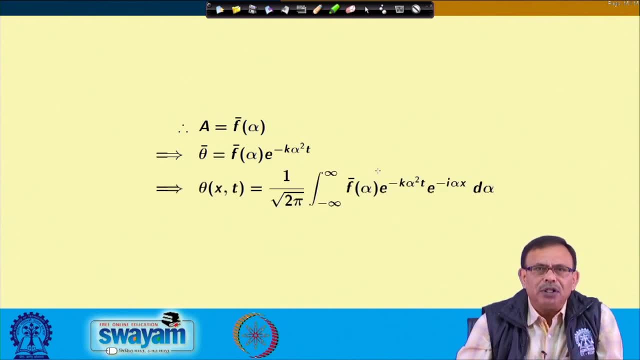 f bar alpha into e power function. So theta t I can write down as an integral like this: and this value is f bar alpha into e power. I can write down this function and once I know the f bar alpha I can tell what is the. 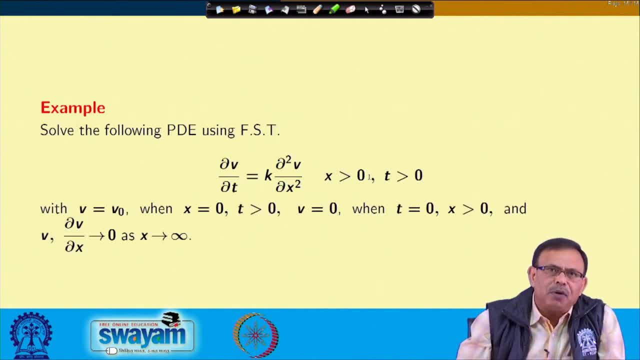 value of theta x, t. Now let us take another problem, this particular problem. earlier, if you remember, we have solved it using Fourier cosine transform. Now the same problem. we want to solve it using Fourier sine transform and we are saying that it is given that v equals v- 0 when x equals 0 and t greater than 0. 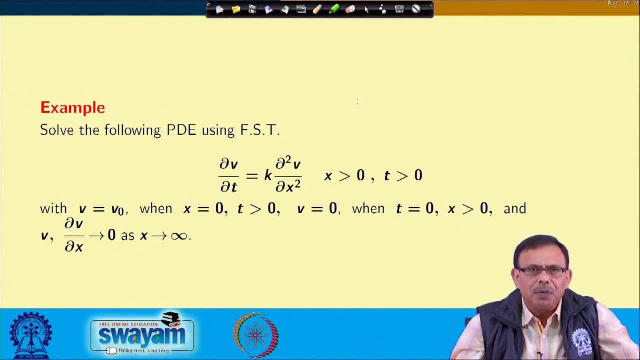 v equals zero when t equals 0 and x greater than 0, and v and del v del x both approaches infinity, both approaches 0 as x approaches infinity. So once I know it from the conditions provided here, and since del v del x approaches 0 as x approaches infinity, I have to take 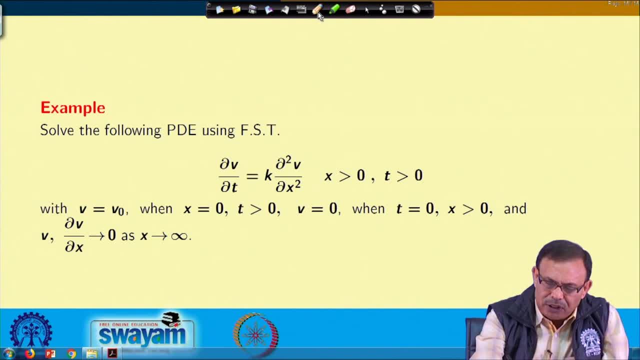 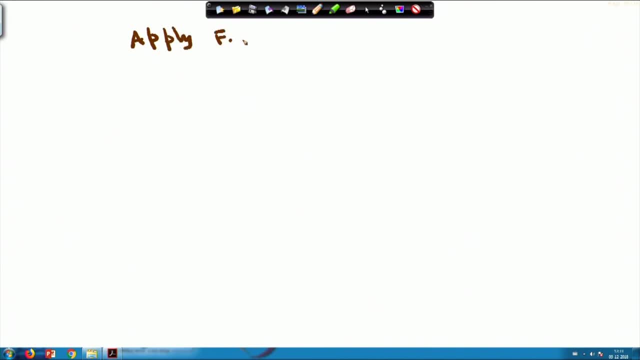 Fourier sine transform with respect to the function x. So let us see this one. So you apply Fourier sine transform with respect to the variable x. So left hand side will be root over 2 by pi 0 to infinity del v del t- was there- del v del t into sin alpha x d. 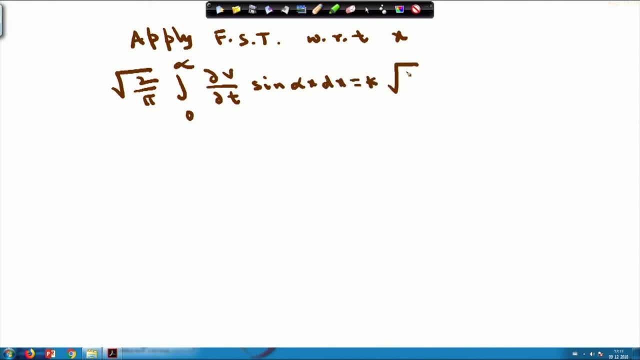 x. This is equals k into root over 2 by pi 0 to infinity, del 2 v, del x square sin alpha x into d x, So that the left hand side will be d d t of nothing but d d t of v bar s. 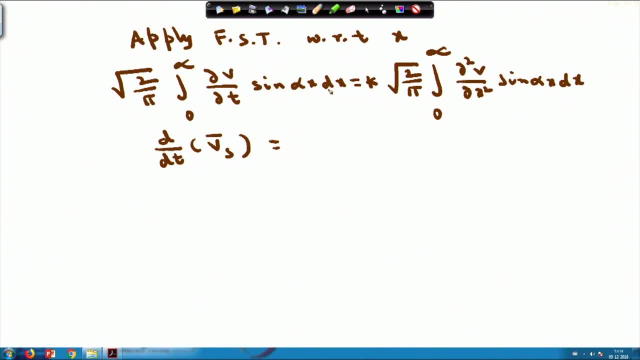 because the integral root over 2 by pi 0 to infinity v sin alpha x, d x is nothing but the Fourier sine transform of v, Which we are denoting as v bar. and this again following the similar process, what we was doing earlier. You will get del v, del x into sin alpha x, 0 to infinity minus alpha, into 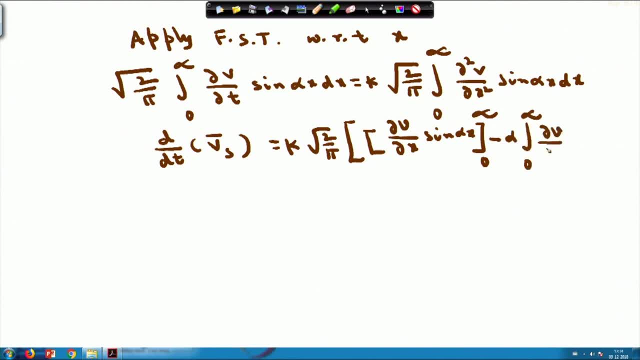 0 to infinity. del v del x into cos of alpha x d x. Again, this first part will be vanishing. So this is equal to del v del x into sin alpha x d x. So this is equal to del v del. 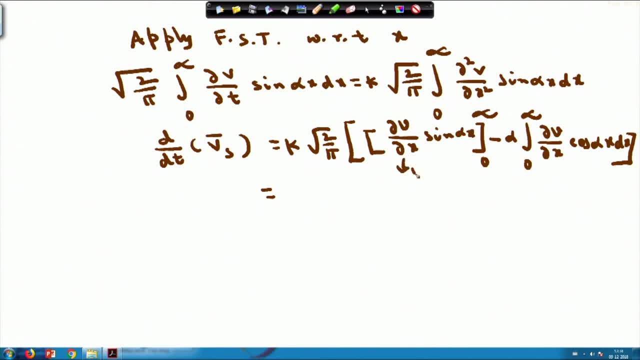 x into sin alpha x d x, because del v del x approaches 0, this approaches 0 as x approaches infinity, So therefore this term will vanish. you will obtain only minus alpha k root over 2 by pi into 0 to infinity del v del x into cos of alpha x d x, And again evaluate this. 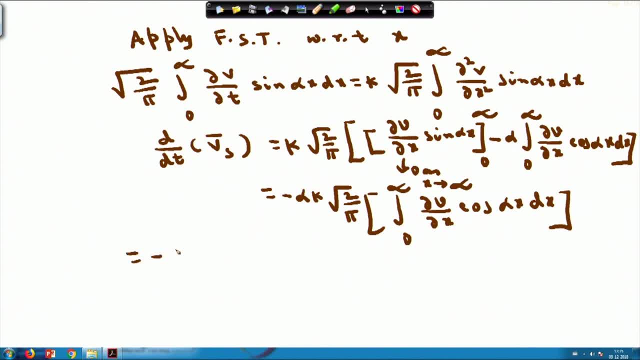 integral. If you evaluate this integral minus alpha x d x, you will get del v del x into sin alpha x 0 to infinity plus alpha 0 to infinity into v sin of alpha x d x plus v sin of alpha x d x. This first part again will vanish, because this one part will vanish. 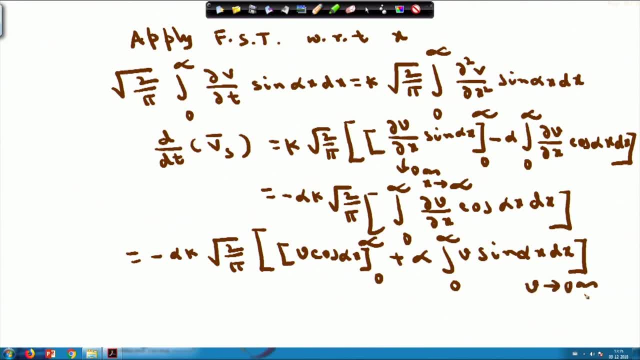 of this. So v approaches 0 as x approaches infinity and v equals v 0 at x equals 0. So that this becomes now will be becoming: first part will be k alpha into v 0, into root over 2 by pi. 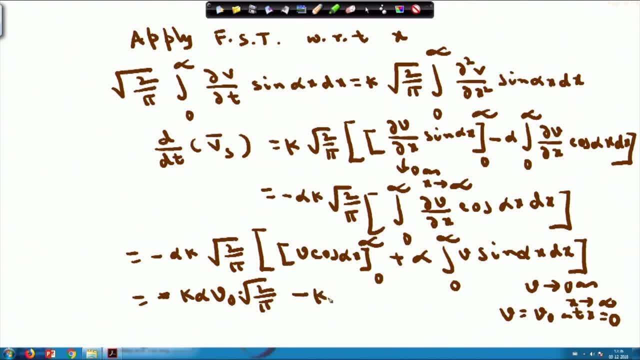 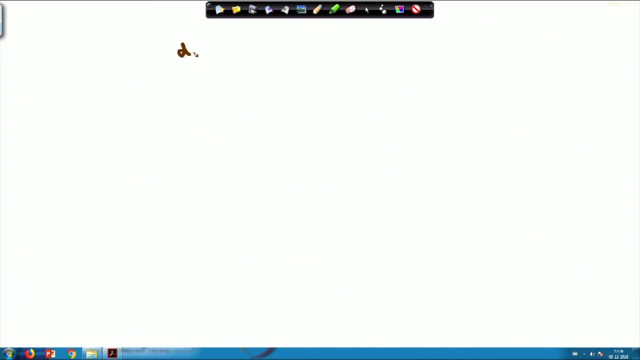 minus this will be k into alpha square, into d bar s. So this part extra term is coming over here now. Therefore, from here the ordinary differential equation, you can write down: d v bar s, d t plus k alpha square v bar s, this is equals. 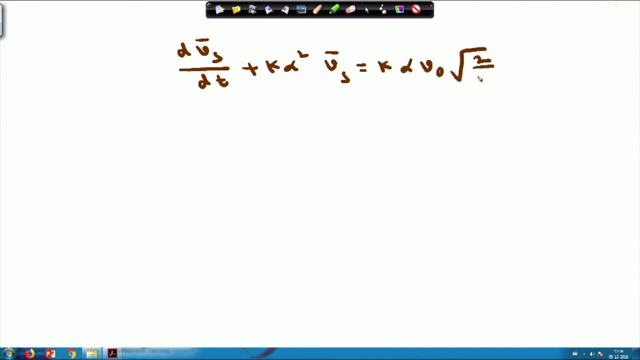 k alpha v 0 into root over 2 by pi. Once I am obtaining this, I am I can write down S into e power k alpha square t. solution of this: C plus root over 2 by pi, V 0 by alpha. 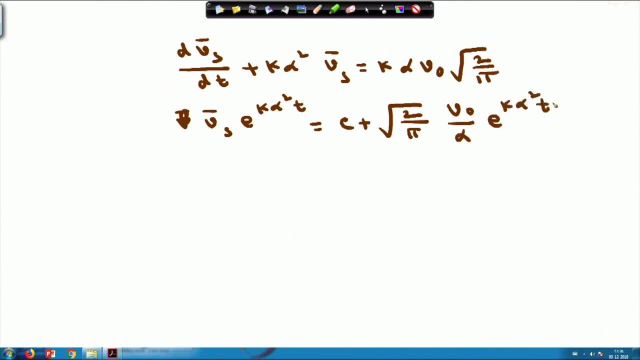 into e, power, k, alpha square t and say: this is your equation 1. Your at t equals 0, your V bar s is 0. This is why, because we know that V equals 0, at t equals 0. This is known to us. Therefore, from here you can tell that V bar s is equals. 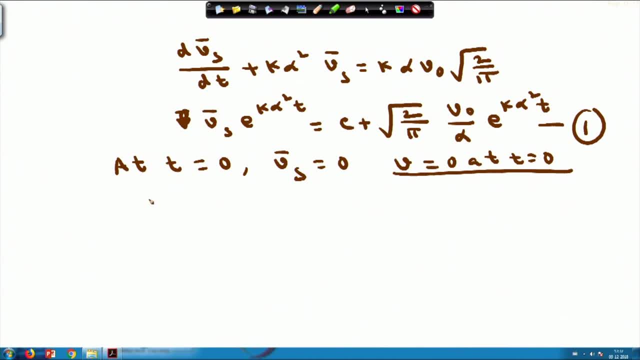 0 at t equals 0. So if you put it in 1, then from 1 what you will obtain 0 equals So C plus root over 2 by pi, V, 0 by alpha. This term also will not be there, So that you: 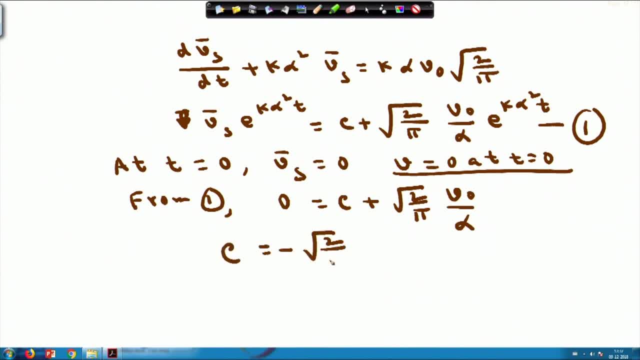 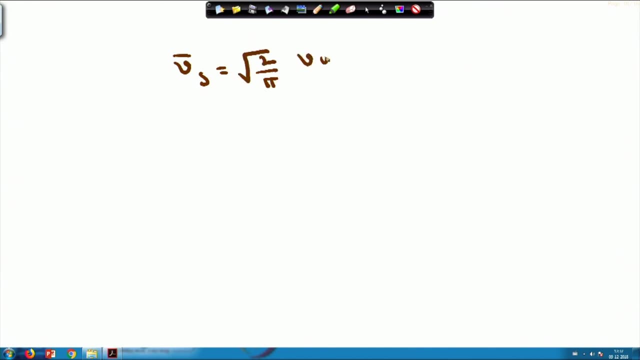 are obtaining the value of C as minus root over 2 by pi into V 0 by alpha. So if I substitute in 1 this value, I will obtain V bar s as root over 2 by pi into V 0 by alpha, into 1. 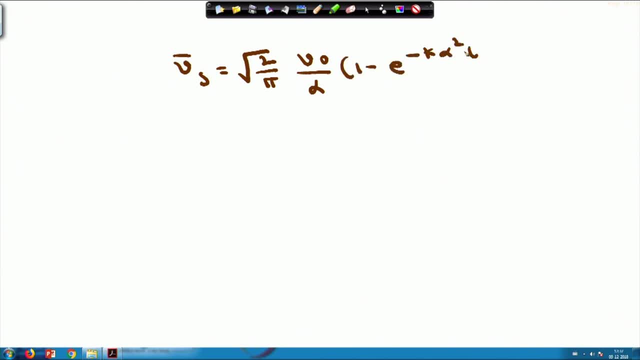 minus e power k alpha square t. So 1 minus e power minus k alpha square into t. and once I have obtained V V bar, in that case I can find out V X t also. This V X t equals 2 by pi. V naught into 0 to infinity. 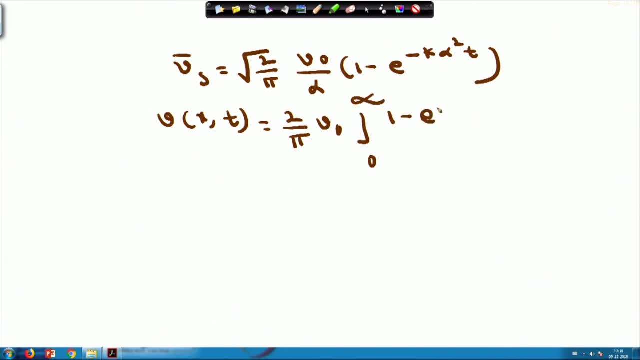 1 minus e power minus k alpha square t by alpha into sine of alpha x into d a plus e d x. This now I can break it into two parts. that is 2 V 0 by pi into 0 to infinity sin of alpha x by alpha into d alpha minus 0 to infinity e power minus k alpha square t by. 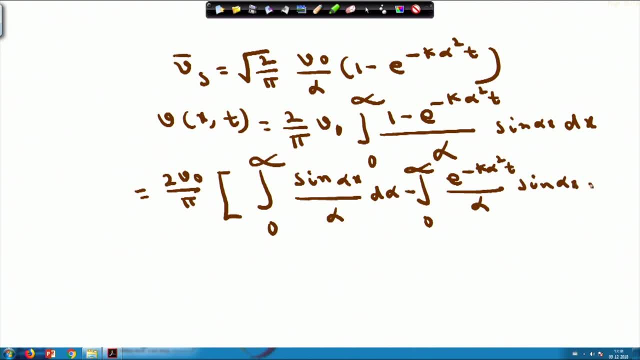 alpha into sin of alpha x into. sorry, this is d alpha, not x, So d alpha. this value is known to us pi by 2, so that this equals. you can write down directly V 0. if I make it, this will be V 0 into this value. is your pi by 2. please note this one. So if it is pi by, 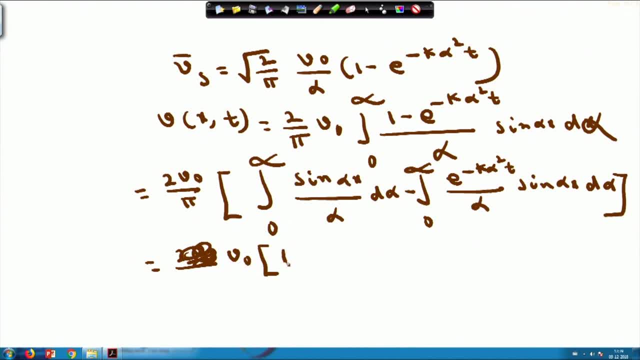 2, this pi by 2.. So pi will be cancelled, so that here there will be 1 minus 2 by pi. please note that this value I have substituted as pi by 2. please note this thing. So this will be becoming: 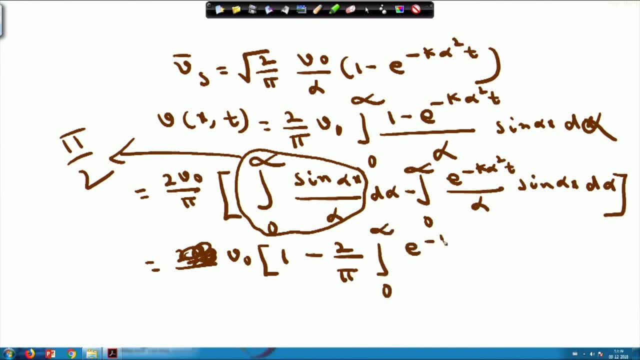 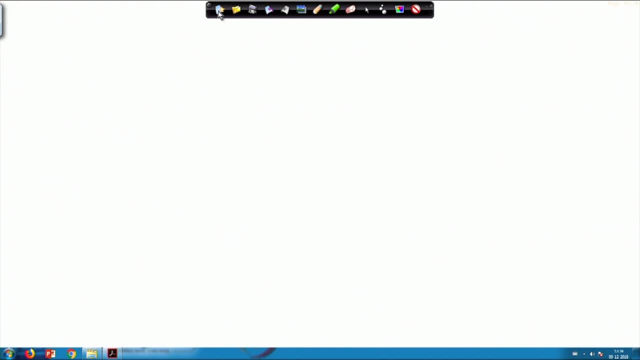 2 by pi 0 to infinity, e power minus k alpha square t by alpha into sin of alpha, x into d alpha. So my next job is to find out the value of this integral. So root over pi by t 0 to x e power minus. 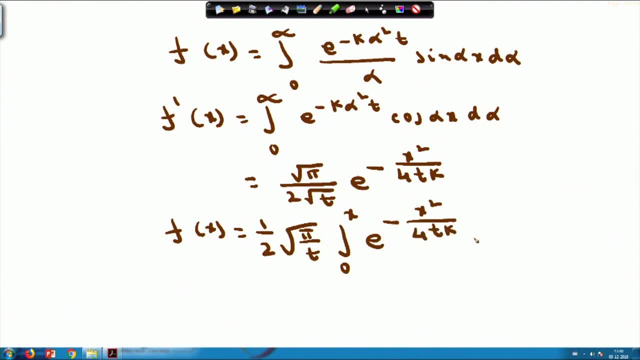 x square by 4 t k into d x and this, if you evaluate again, this equals: you can write down: half into root pi by t into 2 root k t, just some modification. we are making 0 to infinity. my next work: we are making 0 to x e power minus x square by 4 t k into d off x by 2 root. 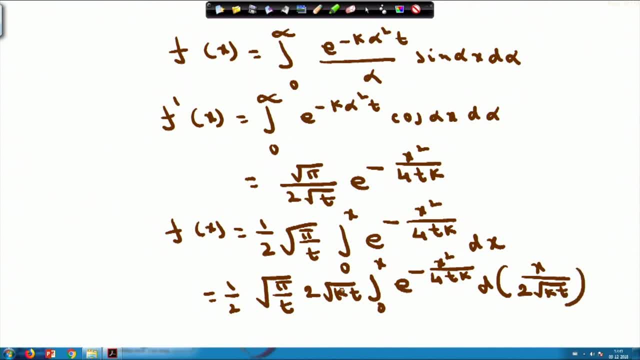 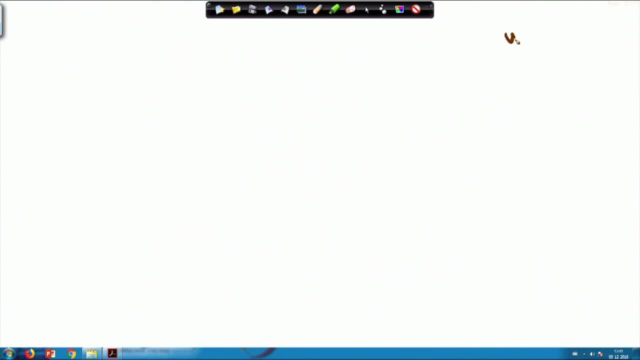 k t. that is the reason this 2 root k t is coming over here. So once I am getting this integral, then on this: if you put u equals x by root over twice kt, you will obtain your f? x as half integral. 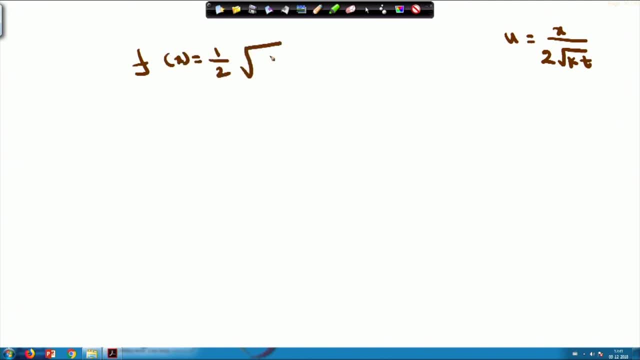 So if I am getting this, So it is e pi rita by k half into root over pi by t into 2 root k t 0 to x by 2 root, x by 2 root t into e power. 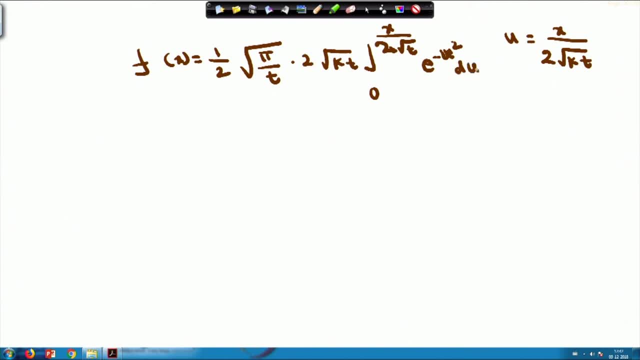 minus u square d? u. Please note this one. This value is known to us and this equals pi by 2 into error function of x by twice root k t. This we have done again earlier. This integral is nothing but e r f of x by 2 root k t, So that your v x t will be equals. 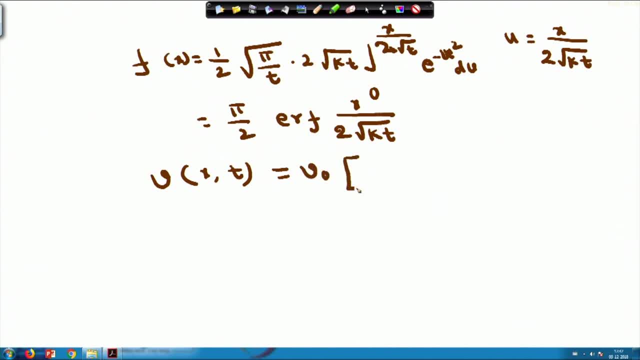 to v 0 into 1 minus e r f of x by twice root k t, And this you can write down: complementary error function. So e r f c of x by twice root k t. So this will be the solution of the given problem. 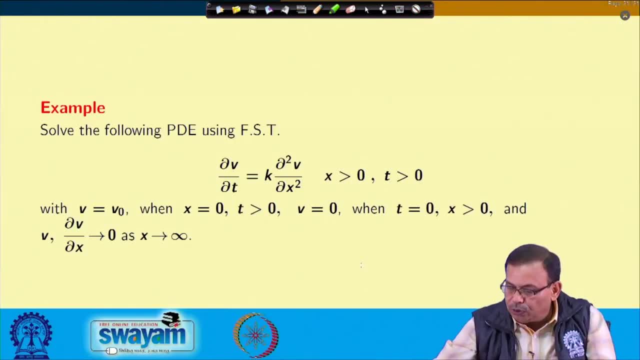 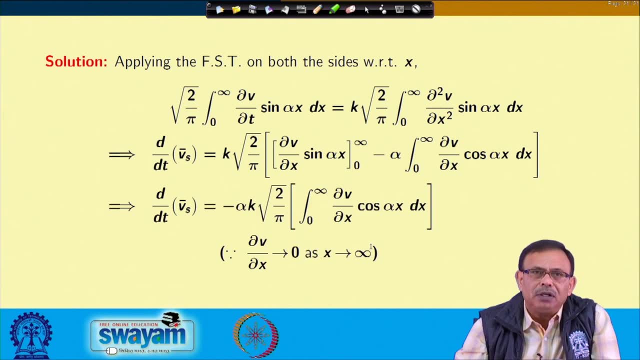 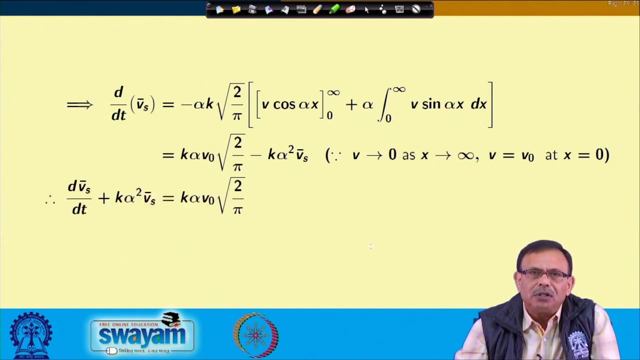 So let us see quickly over here, Once we are getting this, because the solution process is little different. Initial part is same. By this process I am getting the. I am getting by substituting the initial conditions. I am getting the ordinary differential equation. 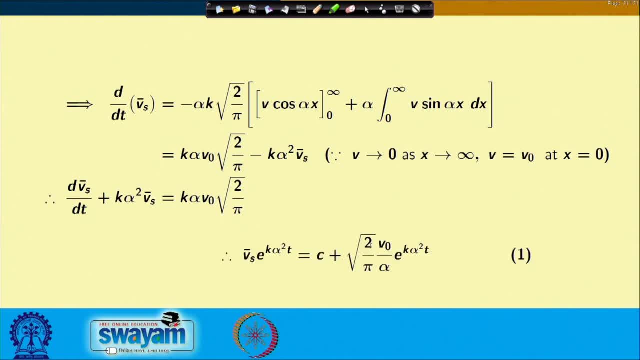 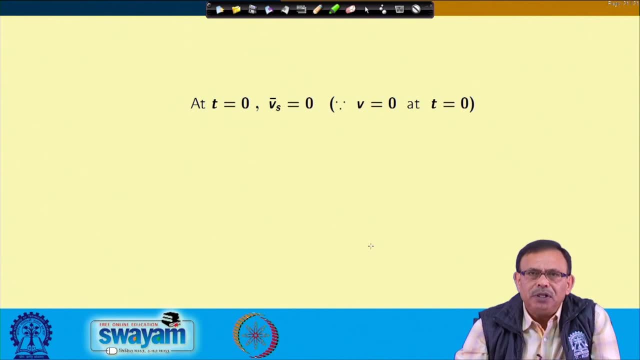 as this, whose solution is written as: v bar s equals this thing, And once I am obtaining this, at t equals 0, v bar s is 0, since v is 0, at t equals 0. So from 1, I can obtain: 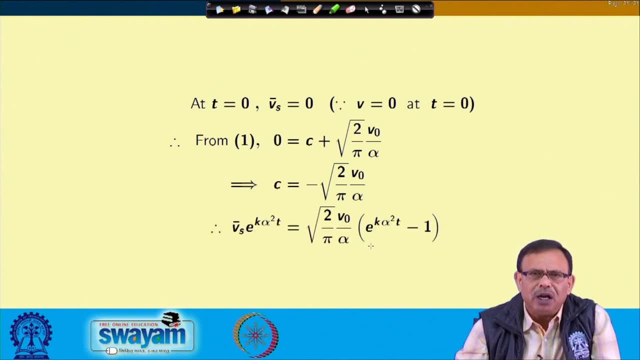 the value of constant c, c. I am getting as this, So that v bar s I am obtaining and v bar s once you are writing, So v x, t, you can write down This. you break it into two parts, two integrals. First integral: 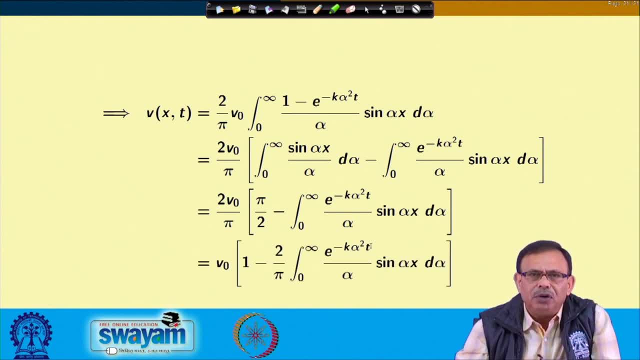 value is pi by 2.. So I am getting v 0 into 1 minus 2 by pi into this integral. My aim is to find out the value of this integral now, which I am assuming as f, x, So that 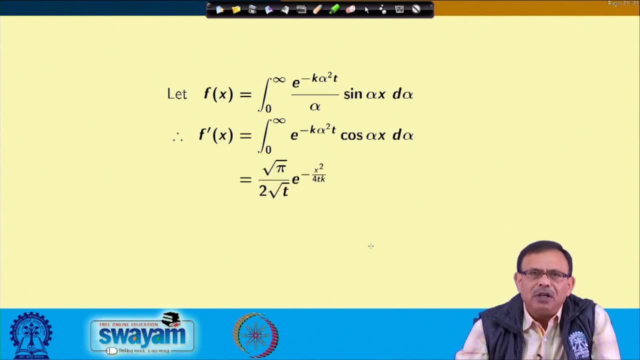 f dash x. from here I can find out, And the value of this integral is nothing but is known to us, the common one. So we have written this so that your f? x will be nothing but half into root over pi.